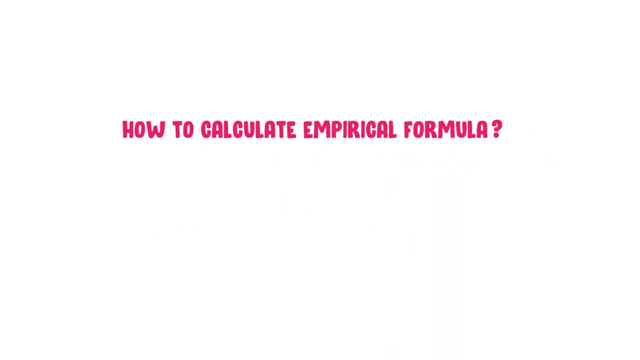 How to calculate empirical formula. I will teach you three most easy steps to calculate empirical formula of any compound. Let's consider that a compound contains 32.65 g sulfur, 65.3 g oxygen and 2.04 g hydrogen. Find its empirical formula. Firstly, I will 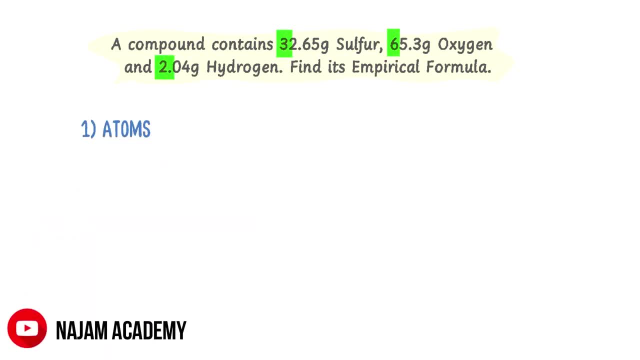 highlight the atoms. For example, there are three atoms given in the question: Sulfur, oxygen and hydrogen. We know that the relative atomic mass of sulfur is 32 g, the relative atomic mass of oxygen is 16 g and the relative atomic mass of hydrogen is 1 g. 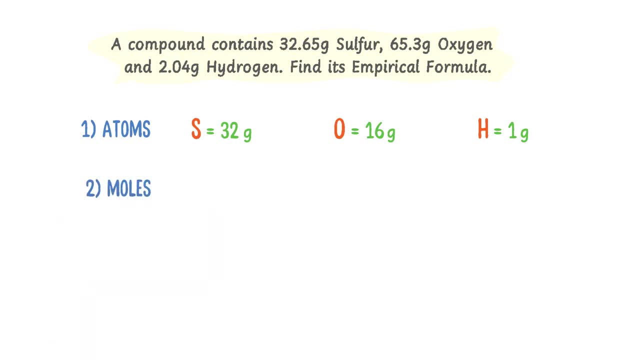 Secondly, I will calculate the number of moles of given elements. It is very easy to calculate. For example, the given mass of sulfur is 32.65 g and I divide it by the relative atomic mass of sulfur, which is 32 g. 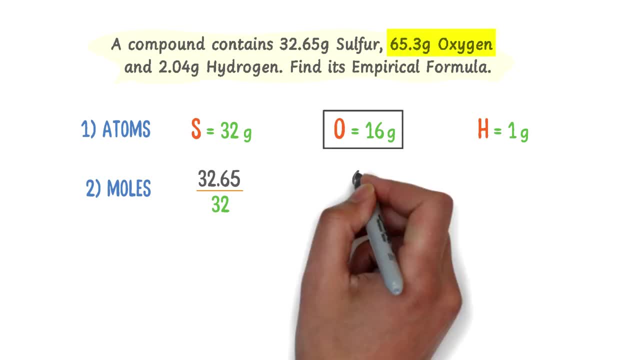 Similarly, I divide the given mass of oxygen, 65.3 g, by the relative atomic mass of oxygen, which is 16 g. Also, I divide the given mass of hydrogen, 2.04 g, by the relative atomic mass of hydrogen, which is 1 g. After calculation, I get 1.02 moles of sulfur, 4.08 moles of oxygen. 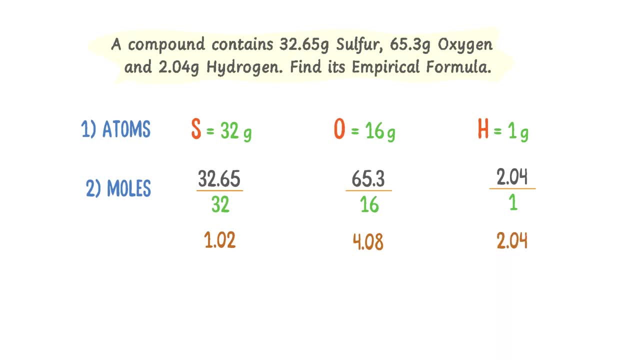 and 2.04 moles of hydrogen. Thirdly, I will find the simplest whole number ratio. To find it, I divide all these three numbers by a smallest number among these three numbers. We can see that the smallest number is 1.02.. So I divide all these three numbers by 1.02.. 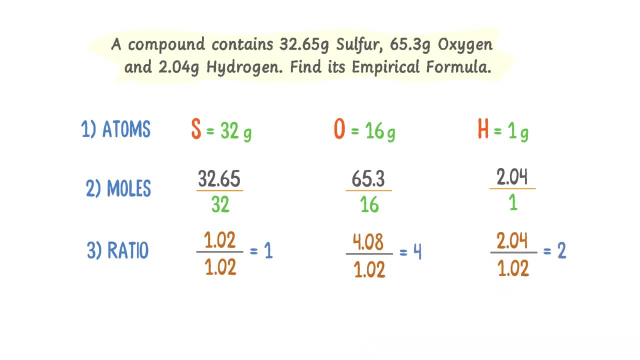 After calculation I get 1,, 4, and 2.. Thus the ratio of sulfur is 1,, the ratio of oxygen is 4, and the ratio of hydrogen is 2, and the compound, Therefore the empirical formula of the compound. 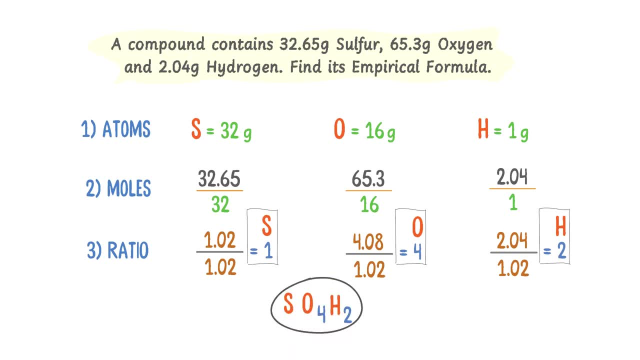 should be SO4 and O2.. Also noted down that in this type of numerical mass composition of elements are given like 32.65 g of sulfur, 65.3 g of oxygen and 2.04 g of hydrogen. 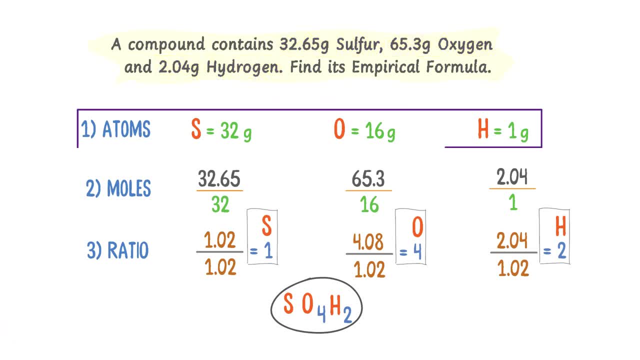 We can calculate its empirical formula by highlighting the atoms and the their relative atomic masses. Secondly, we find the number of moles of these given elements. Thirdly, we calculate the simplest whole number ratio of the elements. Thus, by these three methods, 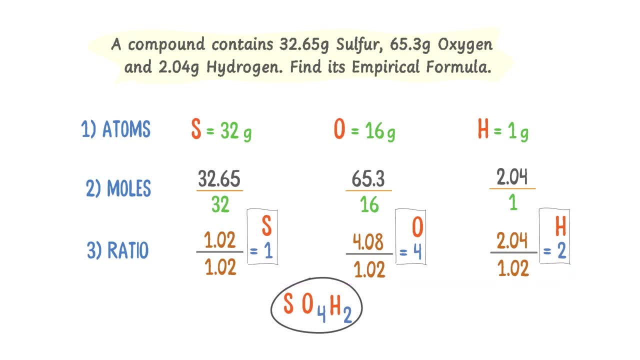 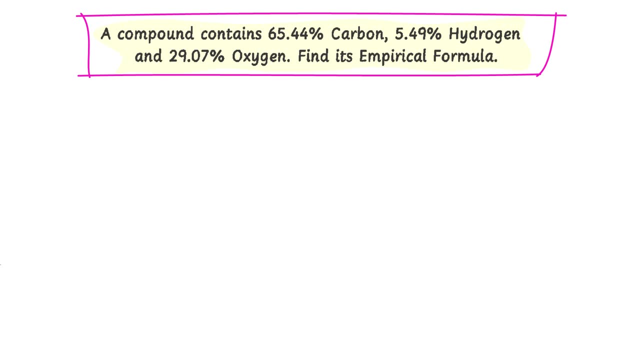 we can easily find the empirical formula of any compound. Finally, let's consider that a compound contains 65.44% carbon, 5.49% hydrogen and 29.07% oxygen. We can also find its empirical formula Here in this type of numerical percentage composition of: 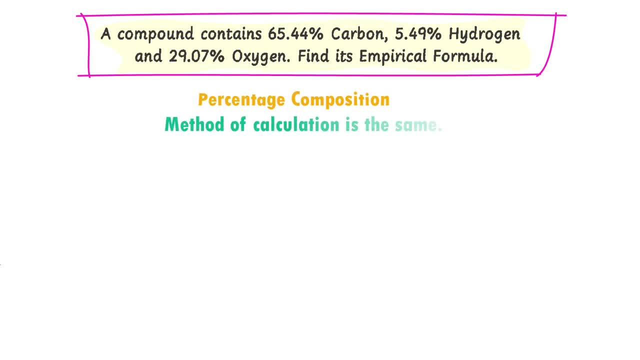 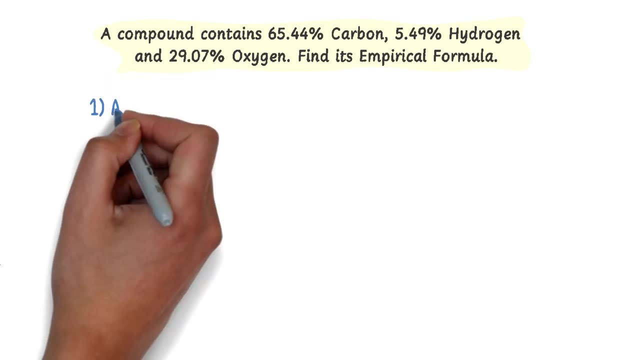 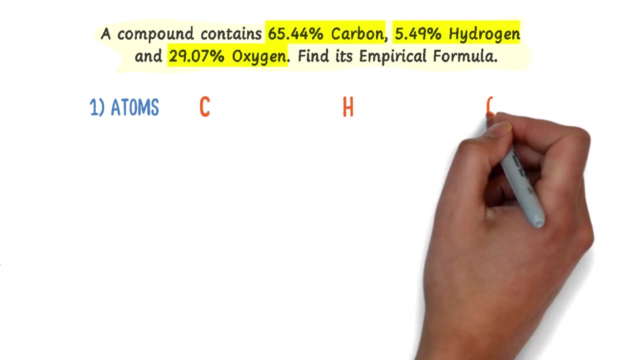 elements are given. Remember that the method of calculating empirical formula from mass composition or percentage composition is the same. So firstly I will highlight the given atoms. For example, there are three atoms given in the question: Carbon, hydrogen and oxygen. We know that the relative atomic mass of 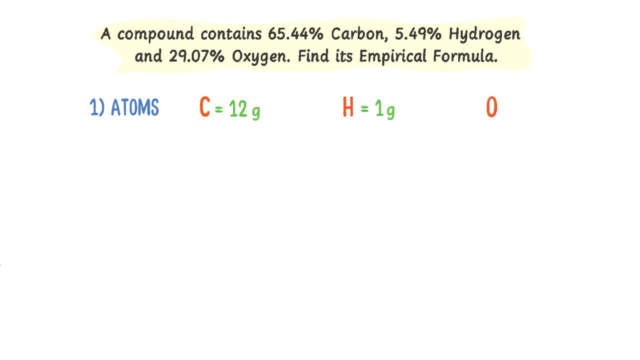 is 12,, the relative atomic mass of hydrogen is 1, and the relative atomic mass of oxygen is 16.. Secondly, I will calculate the number of moles of elements- For example, the given percentage of the carbon is 65.44- and divide it by its relative atomic mass, which is 12.. The given 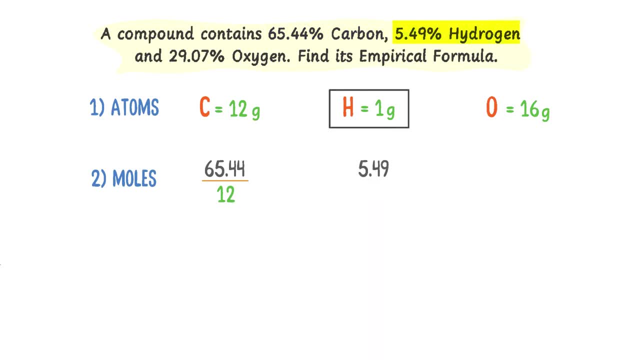 percentage of the hydrogen is 5.49 and divide it by its relative atomic mass, which is 1.. Lastly, the given percentage of the oxygen is 29.07 and divide it by its relative atomic mass, which is 16.. After calculation, I get 5.45 moles of the carbon, 5.49 moles of the hydrogen. Thirdly, I will calculate the 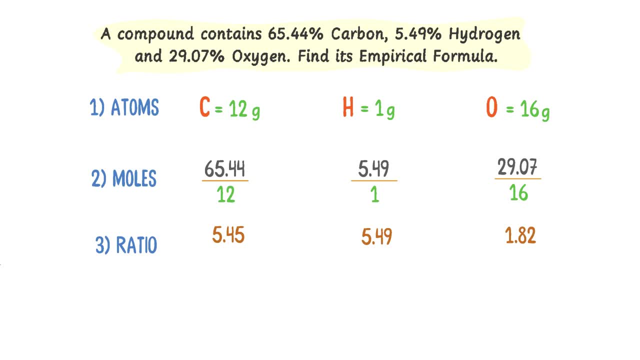 simplest whole number ratio of the elements by dividing all these three numbers by the smallest number, which is 1.82.. After calculation, I get 2.99,, 3.016, and 1.. Now, round about, we get 3,, 3, and 1.. Thus the empirical formula of the compound is C3H3O.